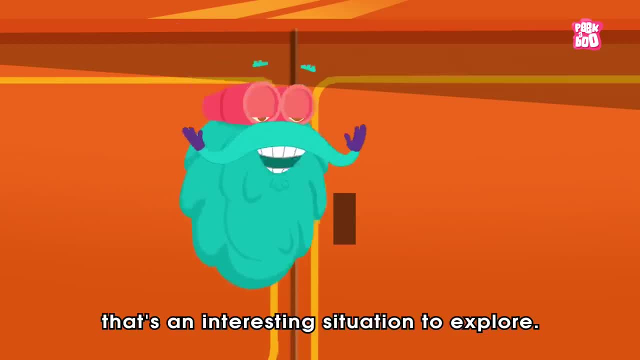 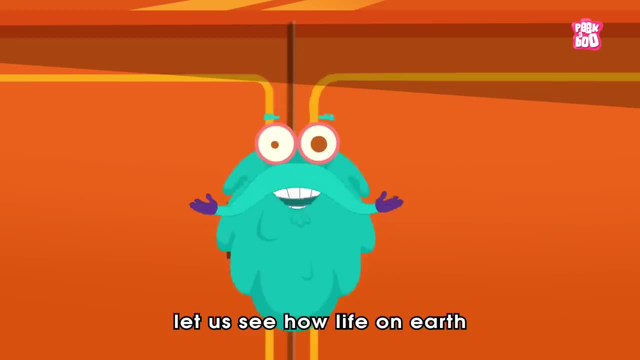 Wait a minute, that's an interesting situation to explore, Hey friends. so in today's episode, let us see how life on earth would be without this powerful force called gravity, And answer a hypothetical question: what if we lost gravity for 5 seconds? 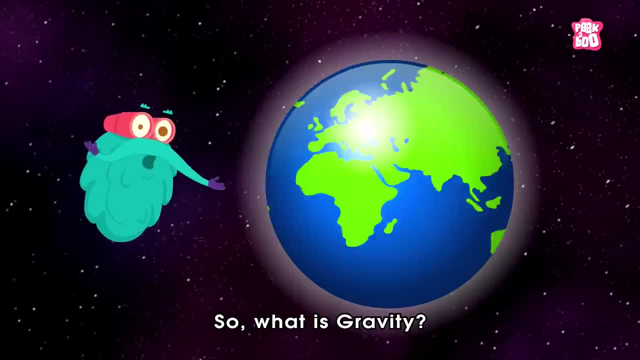 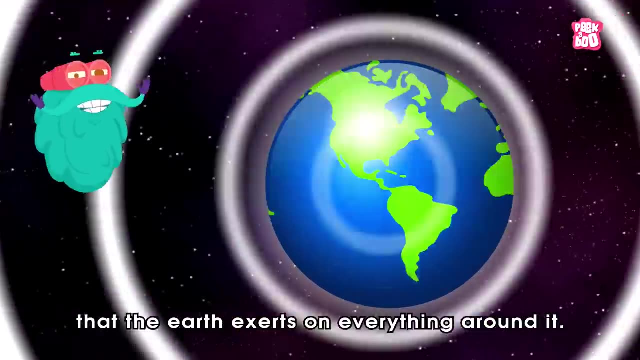 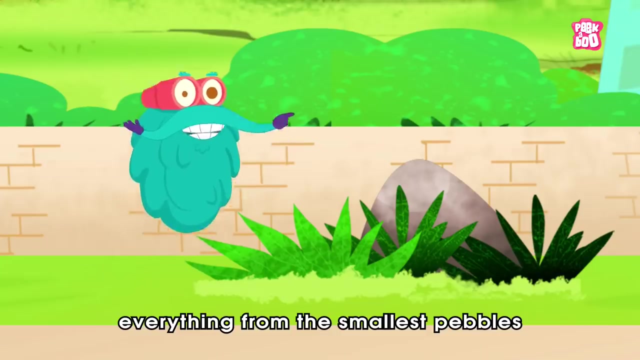 Zoom in. So what is gravity? Well, as we know it, gravity is a force that the earth exerts on everything around it. This includes everything from the smallest pebbles to the tallest skyscrapers. Anything that has mass is in the grasp. 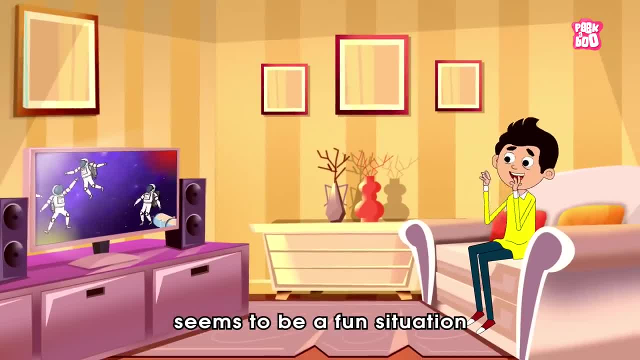 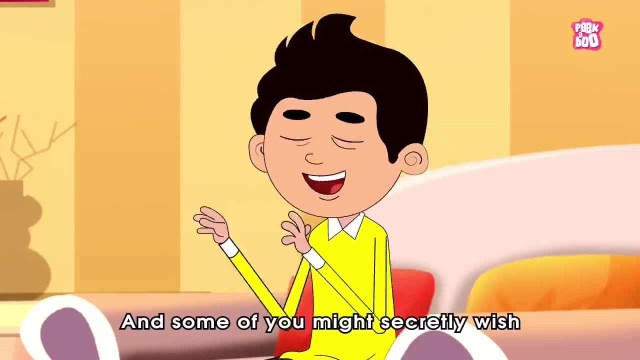 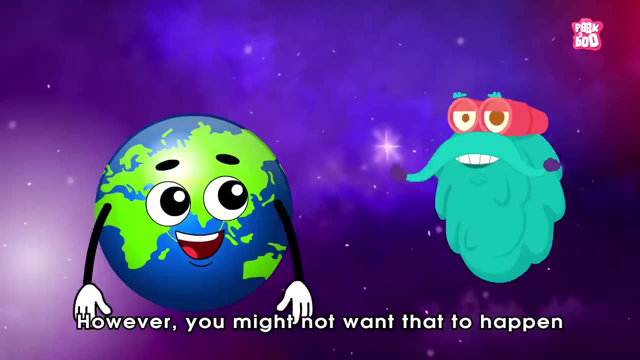 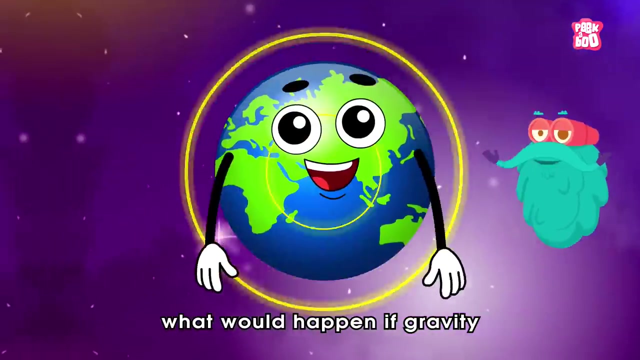 Although the absence of gravity seems to be a fun situation After seeing those astronauts floating in space movies, And some of you might secretly wish for its disappearance so that you can fly freely. However, you might not want that to happen if you fully understood what would happen if gravity ever decides to call it quits. 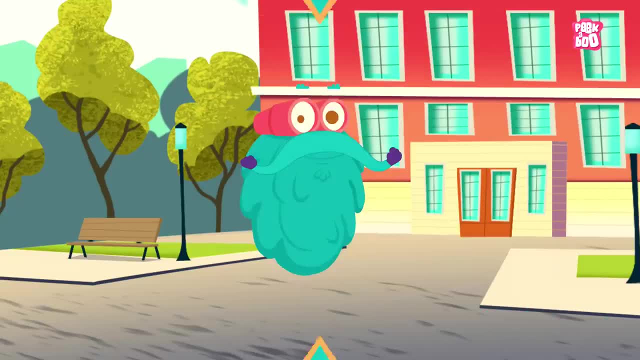 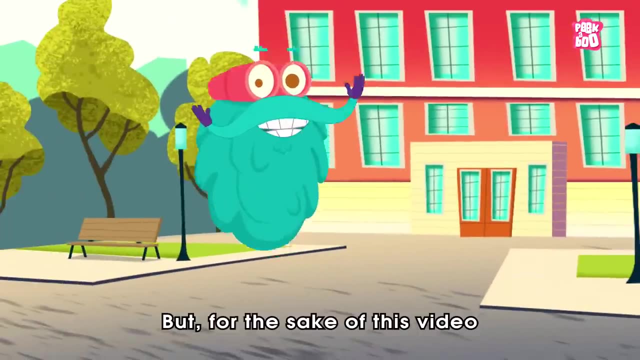 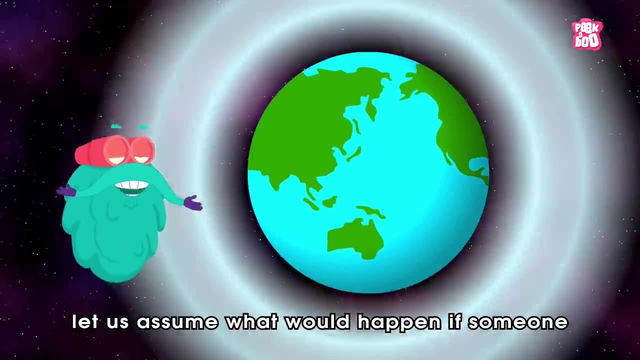 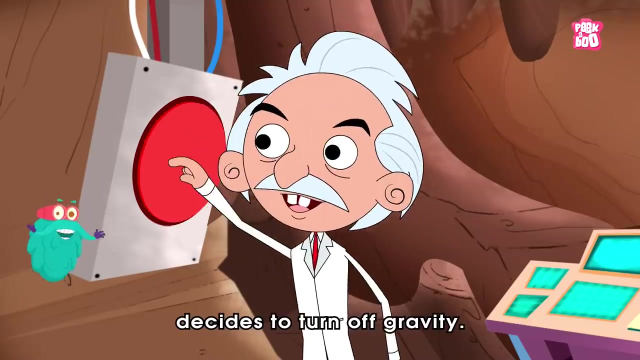 Even for 5 seconds. According to the experts, Such a situation would never, ever occur. But for the sake of this video and to know about the importance of this almighty force, Let us assume what would happen if someone with a desire to fly decides to turn off gravity. 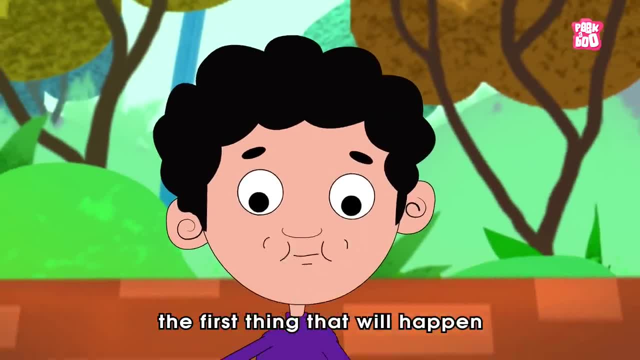 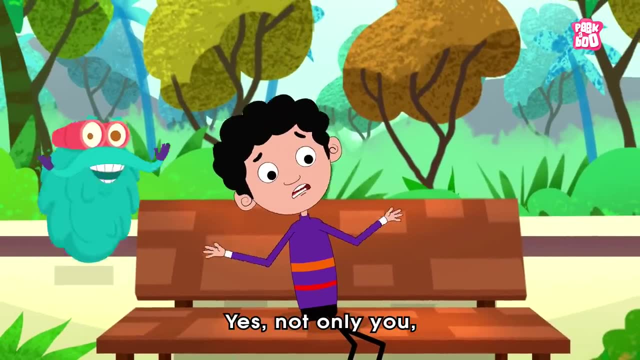 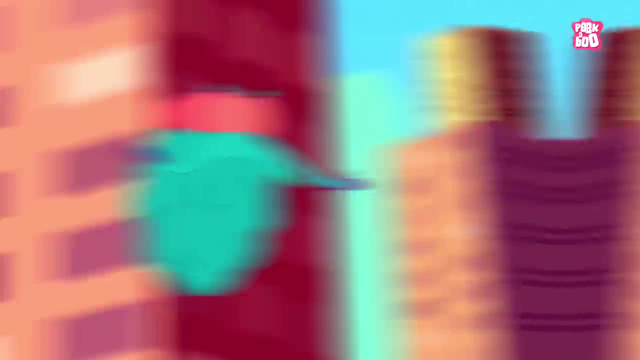 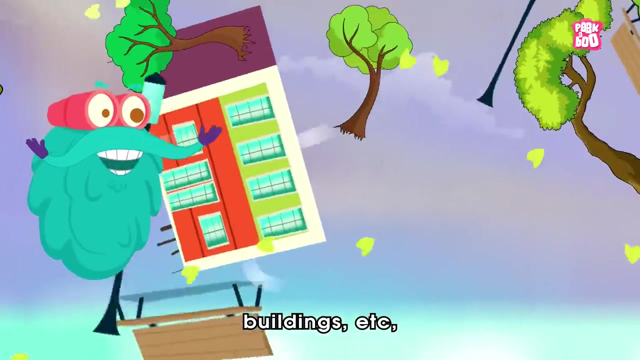 Well, in that case, the first thing that will happen is that everything will go for a toss instantly. Yes, Not only you, but also the vehicles, garbage, animals and so on, Even the things rooted deep inside the ground, like trees, poles, buildings, etc. 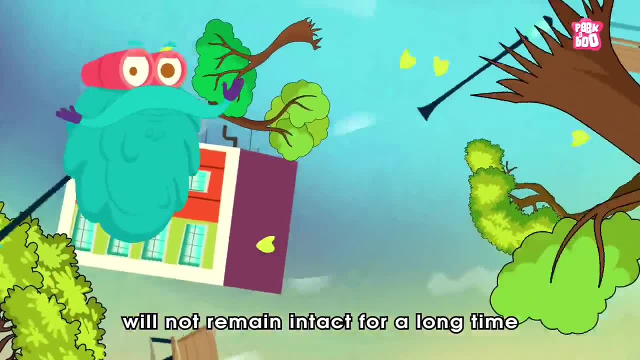 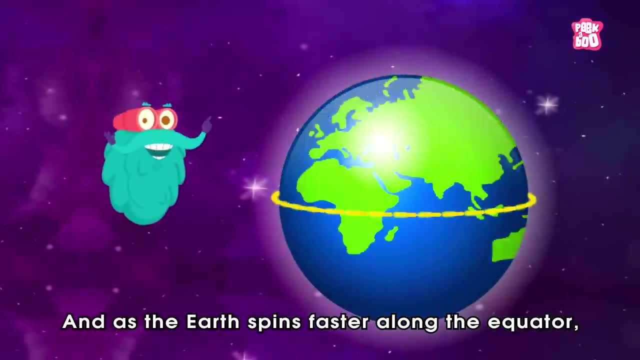 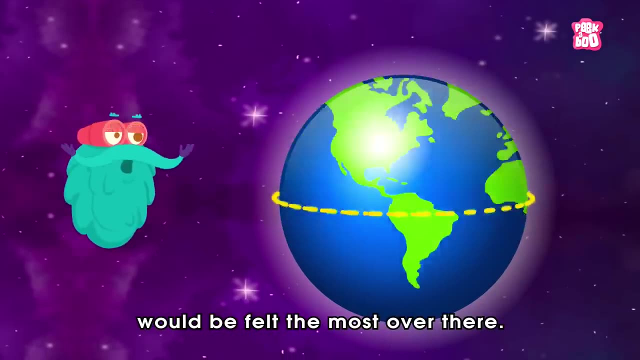 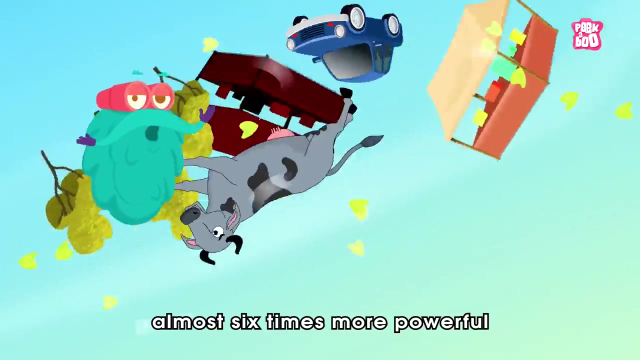 Will not remain intact for a long time and will eventually start tumbling and rolling madly around the earth. And as the earth spins faster along the equator, So the impact of lack of gravity would be felt the most over there. Yes, In the middle of the planet, you could experience winds almost 6 times more powerful than the ones produced by cyclones. 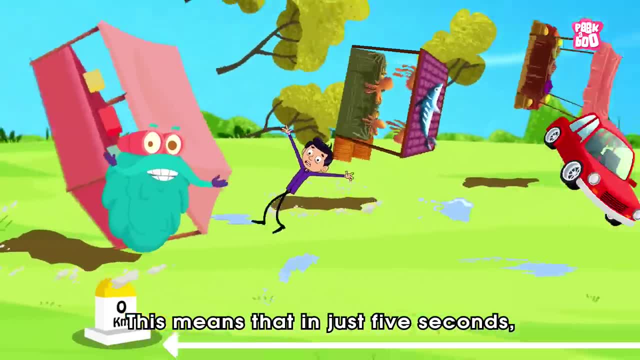 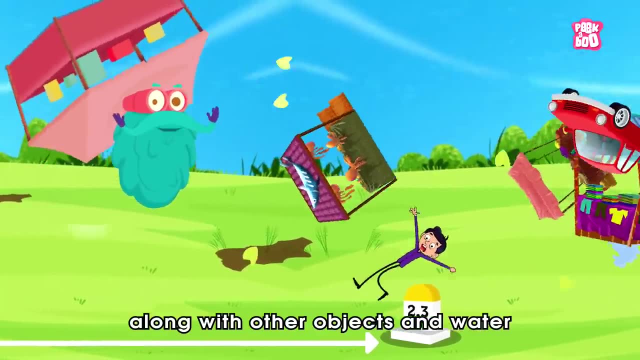 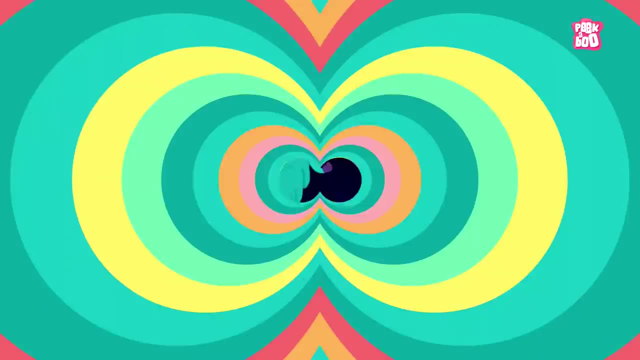 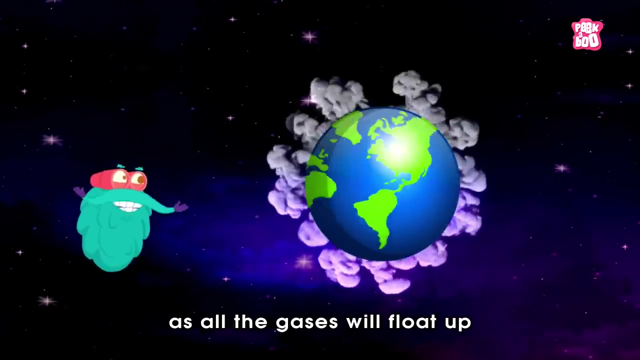 This means that in just 5 seconds, you could be swept as far as 2.3 kilometers in any direction, Along with other objects and water From all the water bodies around the world. Simultaneously, without gravity, the earth's atmosphere would disappear, as all the gases will float up into outer space. 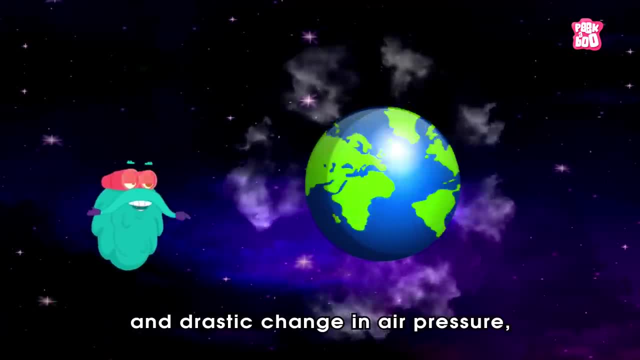 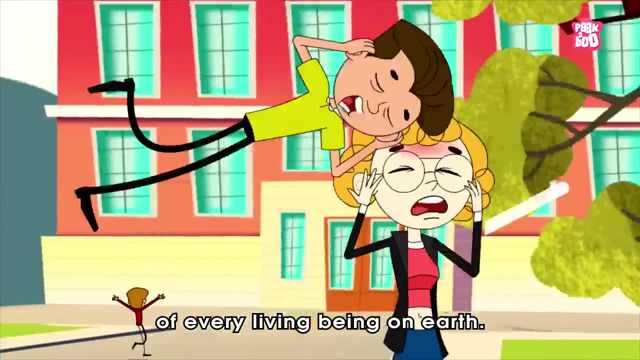 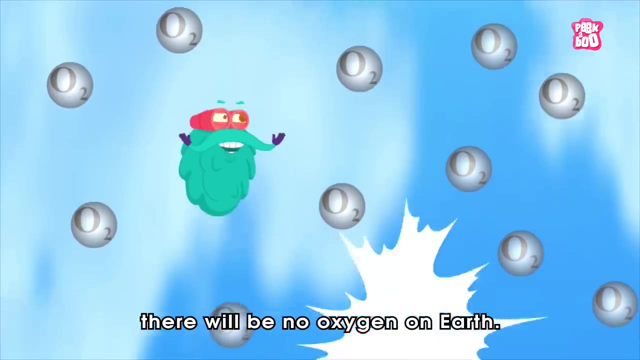 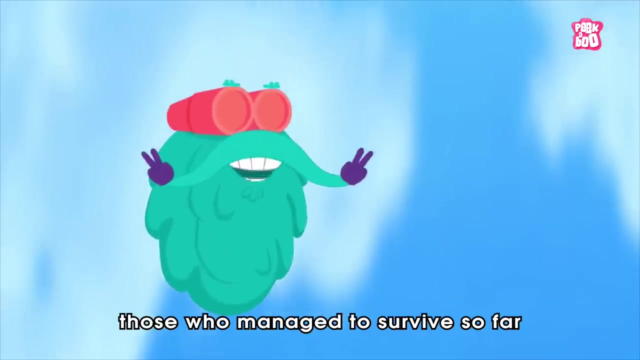 This means that there would be a sudden and drastic change in air pressure Which would immediately rupture the inner years of every living being on earth. Not only that, without the atmosphere, there will be no oxygen on earth, And without the life supporting oxygen, those who manage to survive so far will eventually begin to suffocate, which could be fatal. 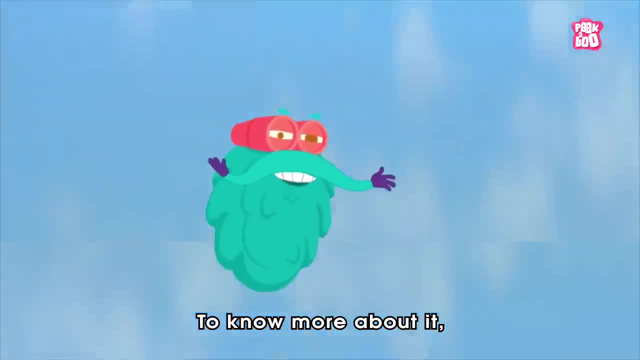 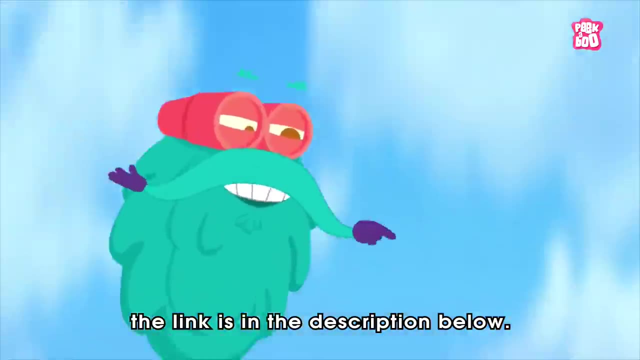 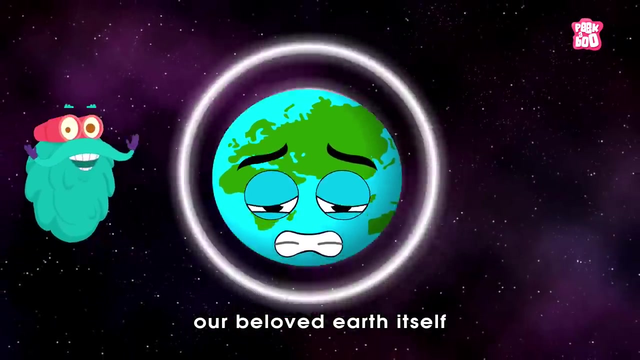 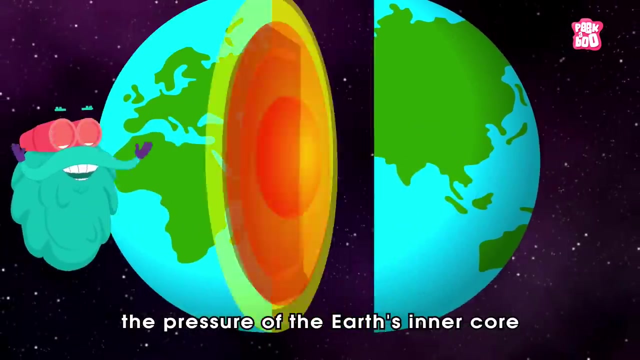 How To know more about it, watch our video. What if the earth lost oxygen for 5 seconds? The link is in the description below. And lastly, as we know, our beloved earth itself is held together by gravity. So without this force, the pressure of the earth's inner core will cause the planet to expand. 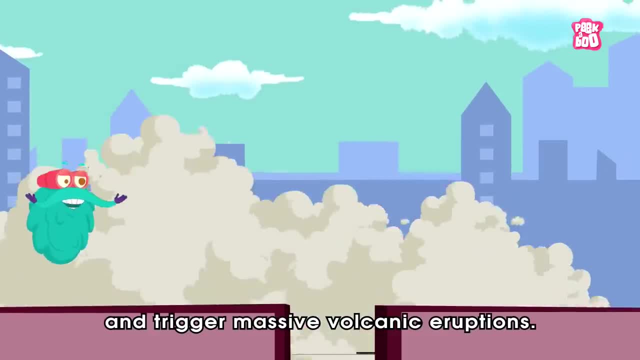 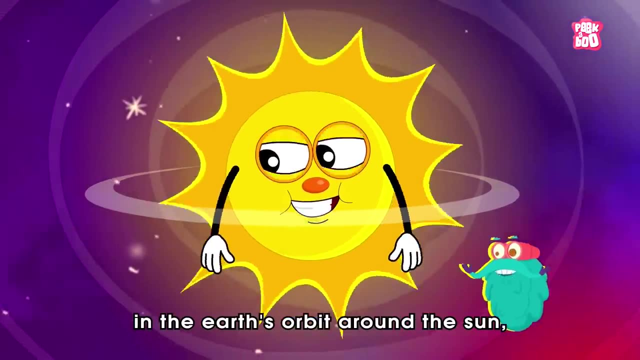 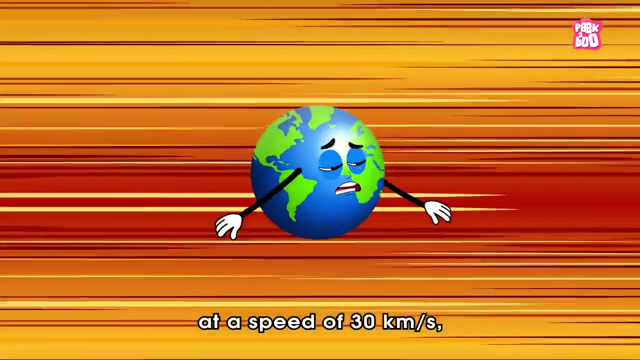 Leading to significant earthquakes and trigger massive volcanic eruptions. And as gravity plays the leading role in the earth's orbit around the sun, It will lose its position and start drifting in space at a speed of 30 km per second, Never to return to the habitable zone. 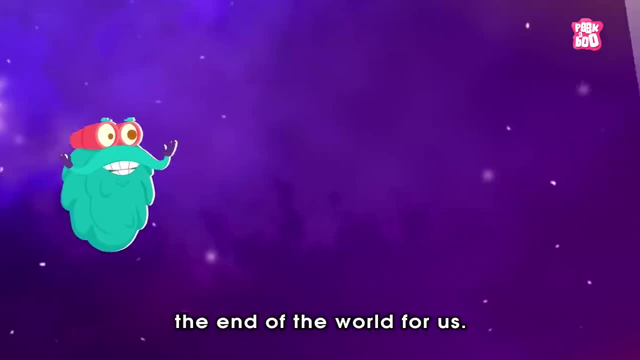 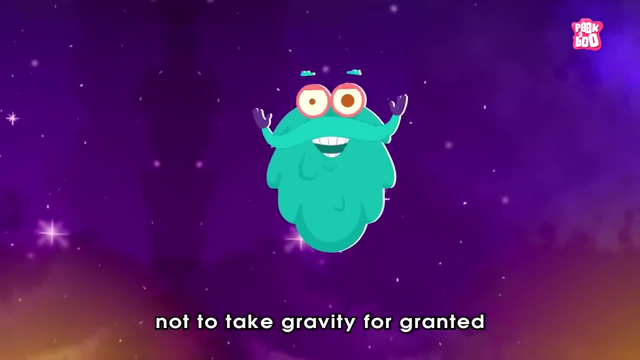 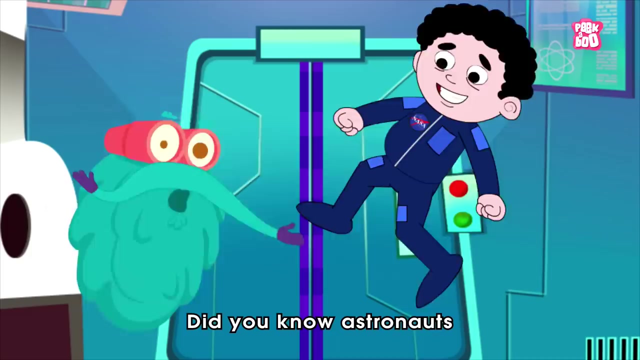 In other words, it will be the end of the world for us. So it's essential not to take gravity for granted and always stay grounded. Trivia time. Did you know Astronauts lose bone mass and muscle strength during stints in space?